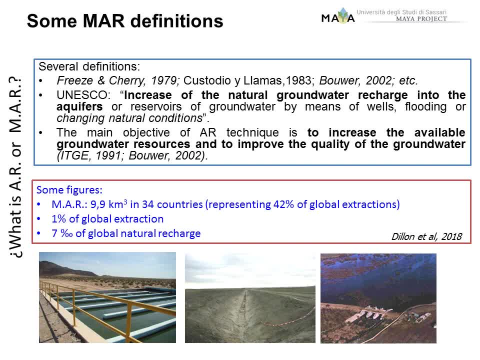 or the one from Bauer, to increase the available groundwater resources and to improve the quality of the groundwater. Whatever be the definition, the most important in my opinion is the word, the keyword. intentional MAR is performed by men, and these figures represent how important this technique is. 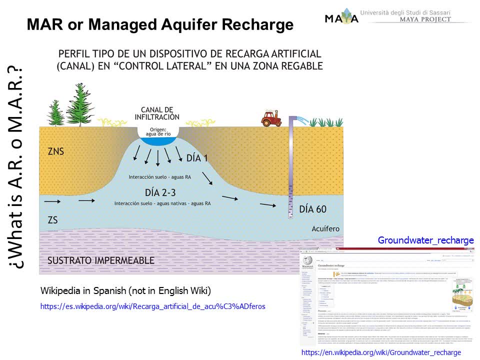 The idea is quite simple. We introduce water either in a point, a line or a polygon. this water progresses across the unsaturated zone until it reaches the groundwater level, and this water already stored is extracted whenever be necessary, either from the same point or from another well or borehole or whatever. 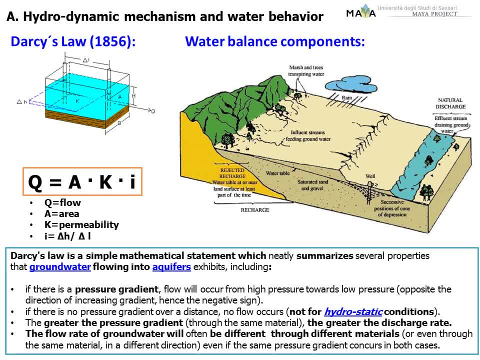 Regarding the hydrodynamic mechanism, there are different formulas, being the most important perhaps Darcy's law, which is a simple mathematical statement which summarizes groundwater flowing into aquifers. It is necessary a pressure gradient. it is not for hydrostatic conditions. 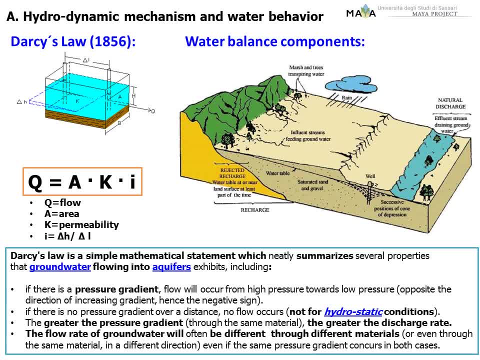 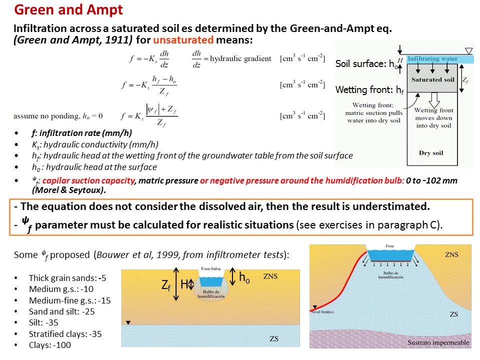 The greater the pressure gradient is, the greater the discharge rate. The flow rate of groundwater will be different through different materials. Sixty years after Darcy Green-Thundam proposed a new formula for unsaturated means in which infiltration rate was a function of the capillary suction capacity. 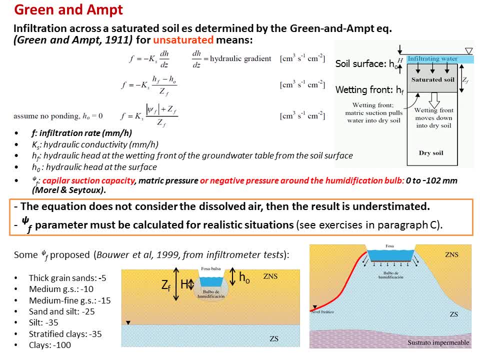 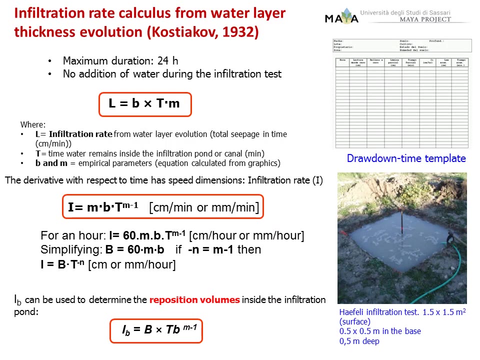 or negative pressure around the humidification valve. This equation does not consider the dissolved air, then the result is underestimated. The phi parameter must be calculated for realistic situations. Later, Kosteykov proposed a new formula for the infiltration rate. 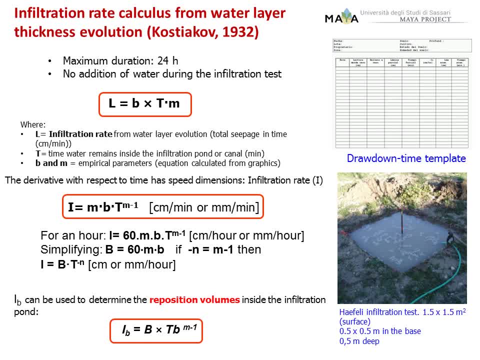 which is a function of the time of the test, and two empirical parameters, b and m. The formula is valid either if there is no addition of water during the infiltration test or there are reposition volumes. It is also usual the use of the Hefele infiltration test. 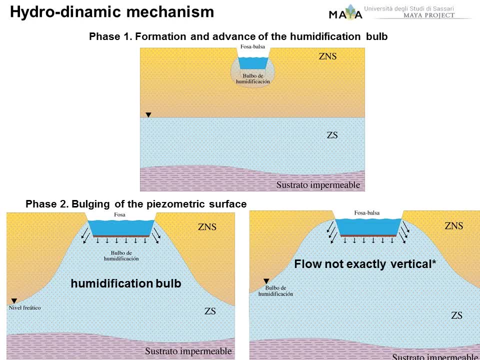 The first phase of the hydrodynamic mechanism is the formation and advance of the humidification valve. The second the bulging of the piezometric surface, where the humidification valve moves across the unsaturated zone with a flow not exactly vertical due to the phi parameter of Green-Thundam. 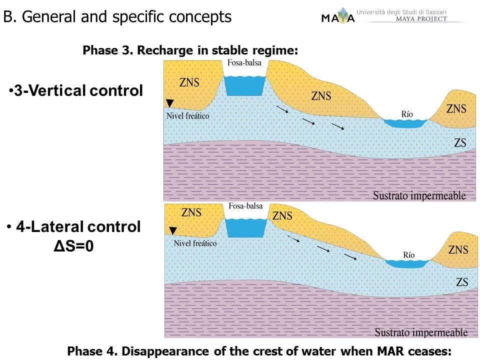 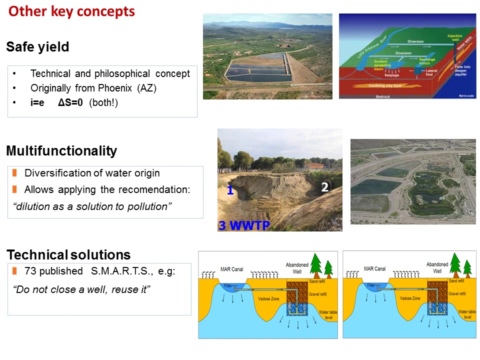 The recharge in a stable regime can work either in vertical control or in lateral control, when the variation of the storage is zero. Finally, when Mars ceases, the crash of water disappears. Some other key concepts are: the safe-yield, a technical and philosophical concept. 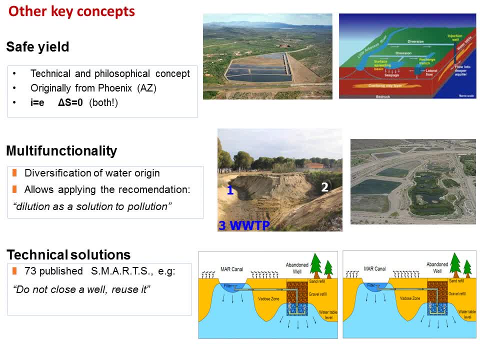 original from Finnish, in which the inflow is exactly the same as the outflow. The multifunctionality is also important. or diversification of water origin. what allows applying the recommendation dilution as a solution to pollution, what means that you can combine different waters from different qualities in different doses. 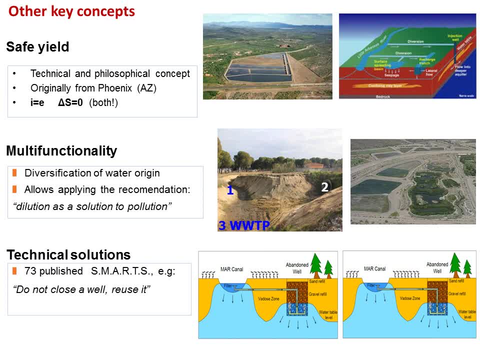 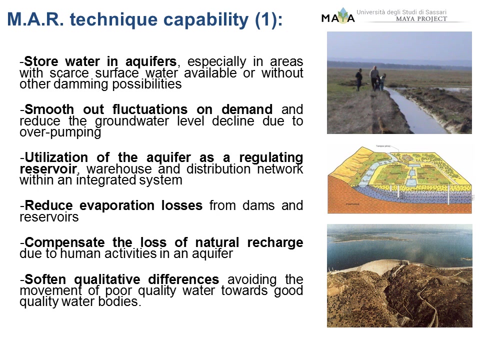 And also it is important to remark technical solutions or sustainable managed-aquifer recharge. technical solutions, For example Dan Klause's well-reused a collection of 73, are published in the references at the end of this lecture. The capability of Mars technique is to store water in aquifers. 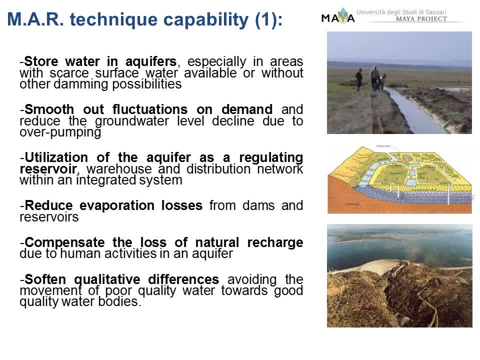 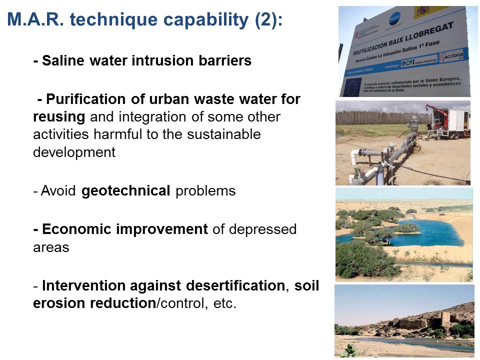 smooth out fluctuations on demand. use of the aquifer as a regulating reservoir. reduce evaporation losses. compensate the loss of natural recharge. soften qualitative differences and thaw water. Saline water intrusion barriers. purification of urban wastewater for reusing. avoid geotechnical problems. 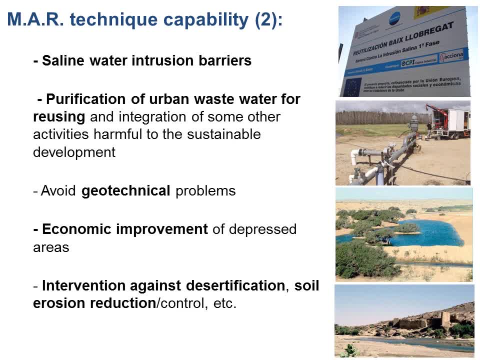 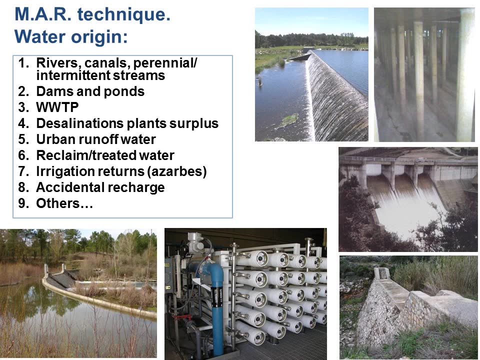 economical improvement of depressed areas and the intervention against desertification, soil erosion reduction, etc. The origin of the water for Mars may be very diverse: either from rivers or canals, perennial intermittent streams, dams and ponds, wastewater treatment plants. 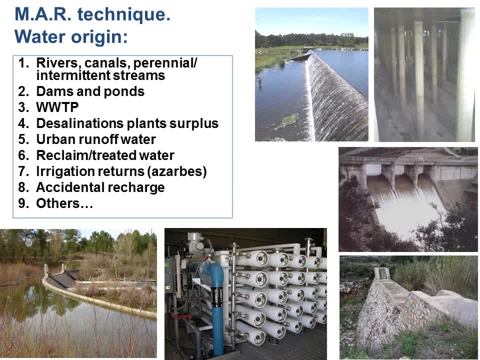 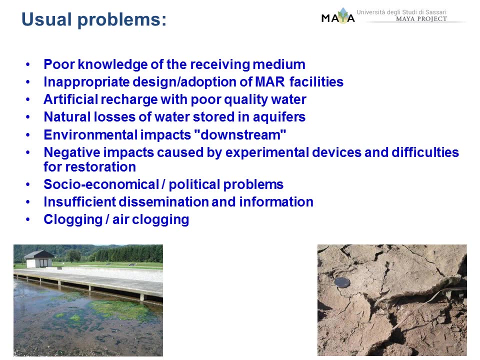 desalination plants, urban runoff water, reclaimed or treated water, irrigation returns, accidental recharge, etc. Some of the usual problems when performing Mars activities are the poor knowledge of the receiving medium, the inappropriate design of Mars facilities, the use of water of poor quality. 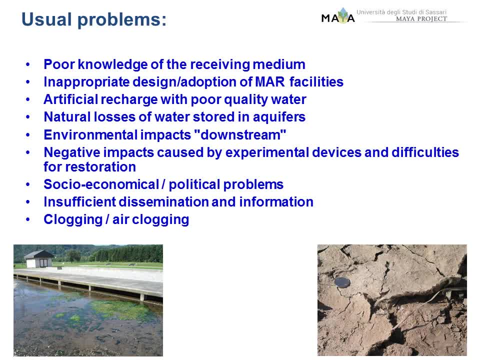 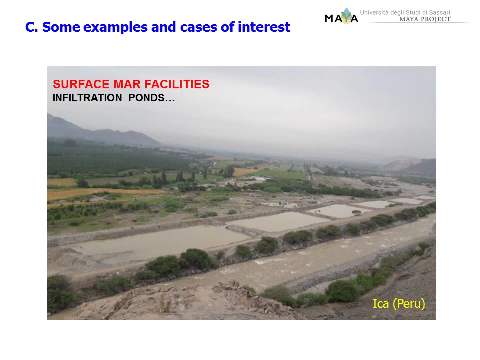 the natural losses of water stored in aquifers, the environmental impacts downstream, some other negative impacts caused by experimental devices, socio-economical and political problems, insufficient dissemination and information of the results and, of course, logging Some examples and cases of interest for surface Mars facilities. 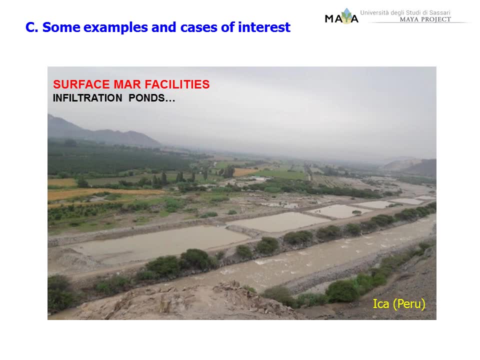 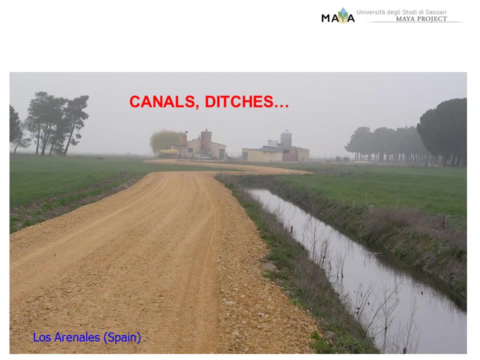 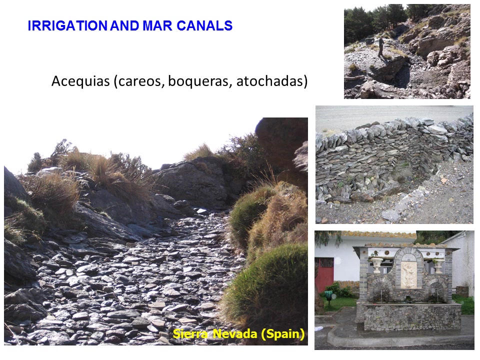 are the infiltration ponds, the most usual Mars facility in the world. this is an example from Nika, Peru. canals and ditches also very spread all around the globe. irrigation and Mars canals, for example, the Careas from ancient times. 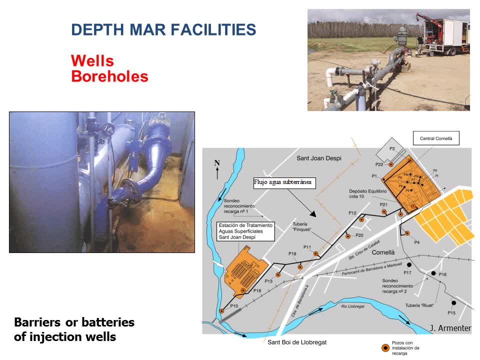 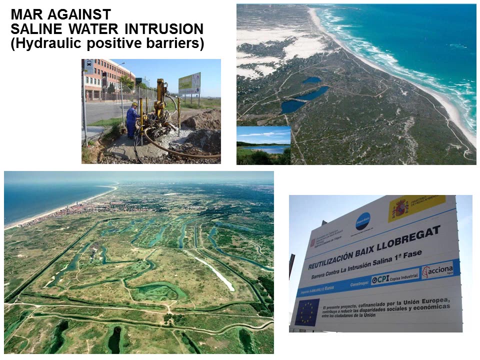 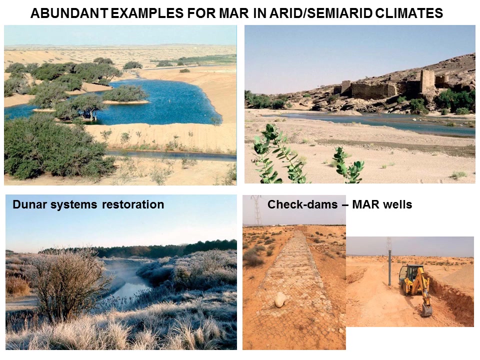 and for deep Mars facilities, it is usual the use of wells, boreholes and barriers or batteries for injection wells. Mars is also used to combat saline water intrusion by means of hydraulic positive barriers, and there are abundant examples for Mars in arid and semi-arid climates. 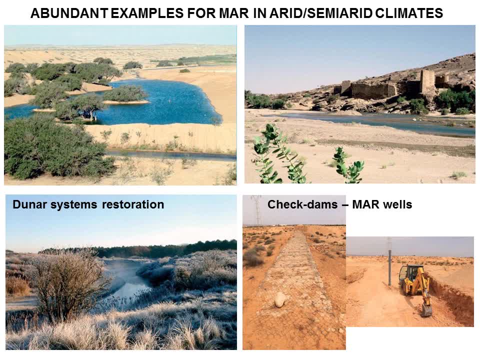 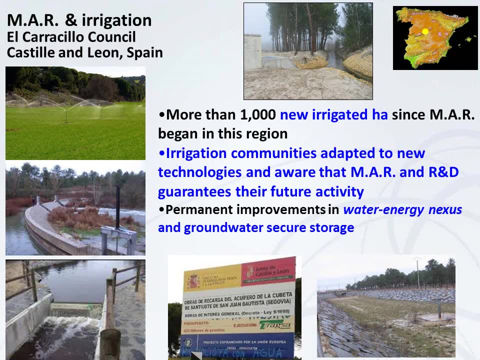 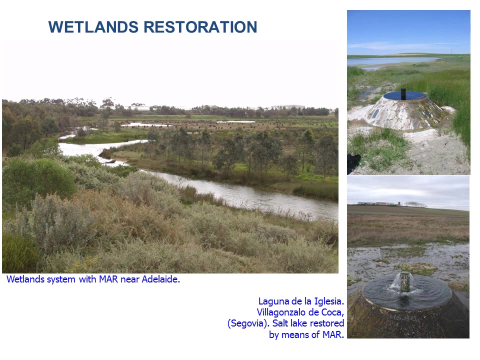 for example, this during our system restoration and the combination of check dams and Mars wells. The most normal use of Mars water is for irrigation. there are permanent improvements in water energy, nexus and groundwater secure storage, and Mars is also used for wetlands restoration, with abundant examples all over the world. 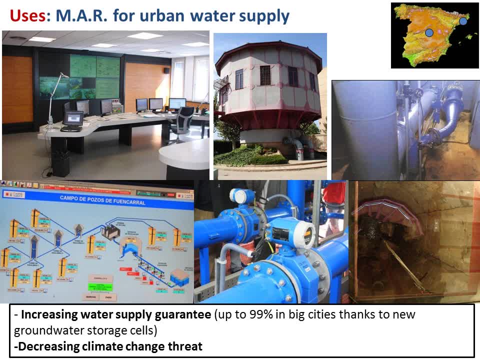 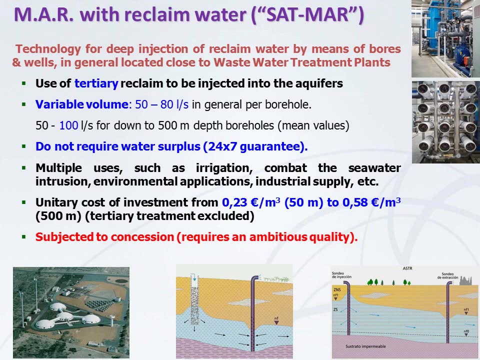 Eventually, Mars is also used for urban water supply, increasing the water supply guarantee and decreasing the climate change threat. Mars with reclaimed water is usually called Sat-Mars, is a technology for deep injection of reclaimed water by means of boards and wells. 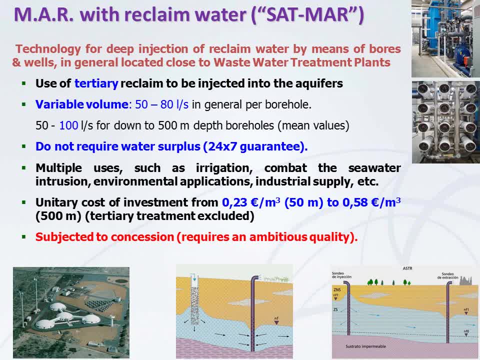 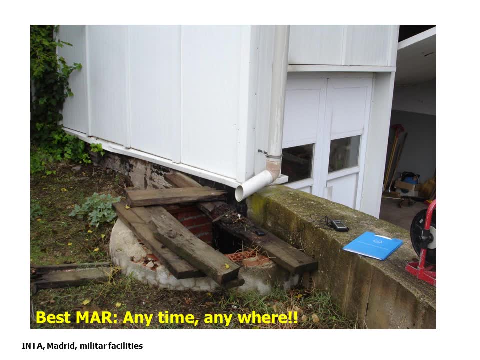 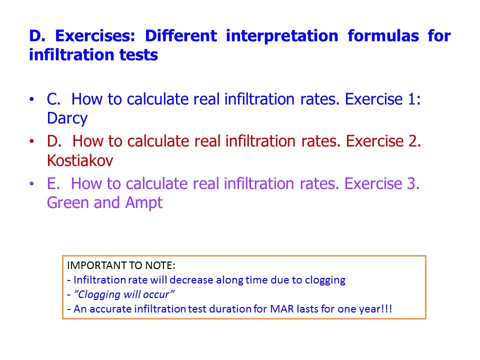 in general located close to the wastewater treatment plants. where water is diverted, It is subjected to concession and requires an ambitious quality. So, in short, Mars Technique presents more pros than cons. It is usual to find problems during the interpretation of infiltration tests. 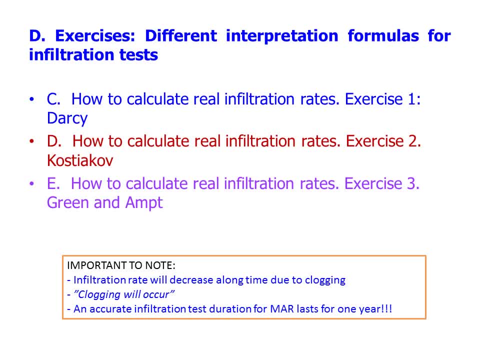 This is why we have proposed a set of three different exercises applying three different methods. It is important to note that infiltration rate will decrease a long time due to clogging. clogging will occur and an accurate infiltration test duration for Mars lasts maybe one year. 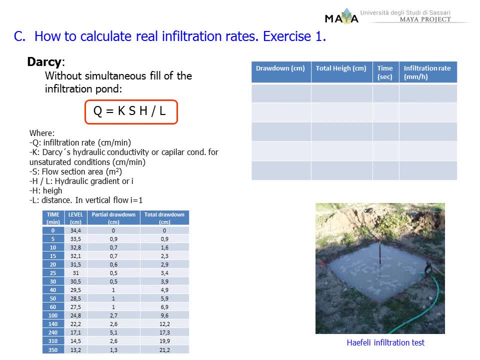 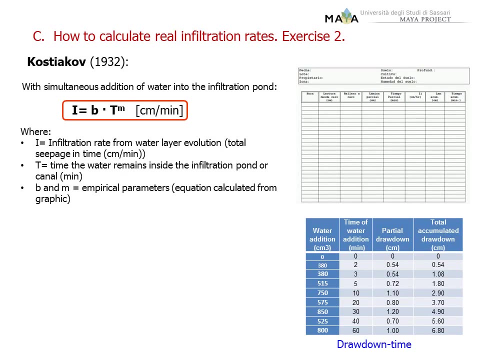 In the first exercise, we are going to use Darcy's law to calculate the infiltration rate from the data collected from the Hefele infiltration test displayed in this template. The second exercise exposes a collection of data gathered from an infiltration test and we will calculate the infiltration rate.